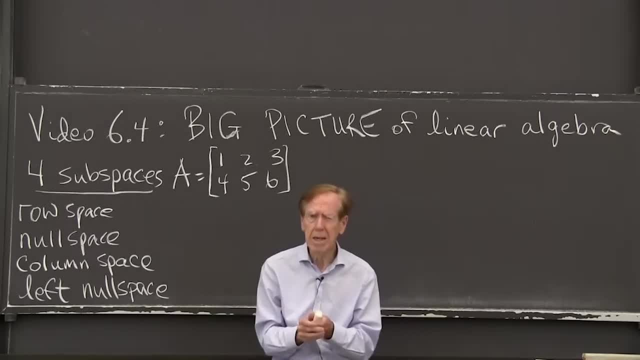 Now if I take all their combinations, do you kind of visualize that if I have two vectors and I add them, then I get another vector that's in the same plane. Or if I subtract them, I'm still in that plane. Or if I take 5 of 1 and 3 of another. 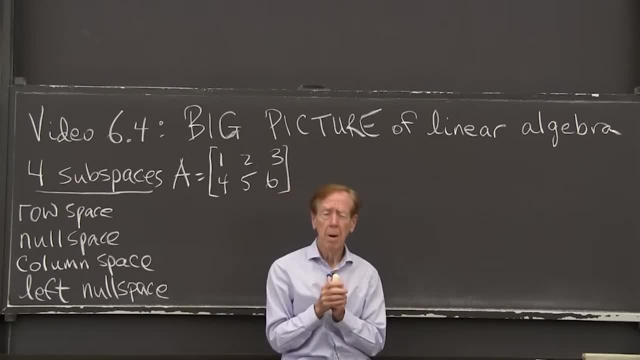 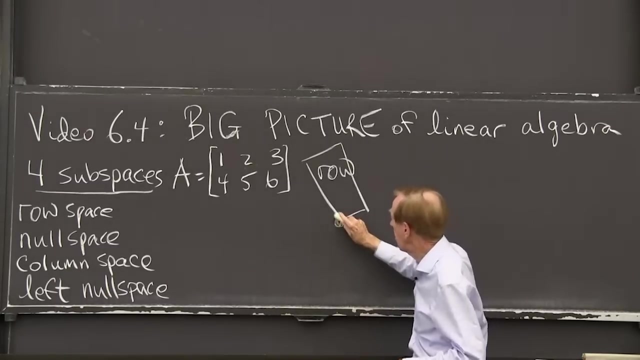 I'm still in that plane And I fill the plane when I take all the combinations. So the row space. can I try to draw a picture here? It's a plane, This is the row space. I'll just put row And in that plane are the vectors 1,, 2,, 3, and the vector 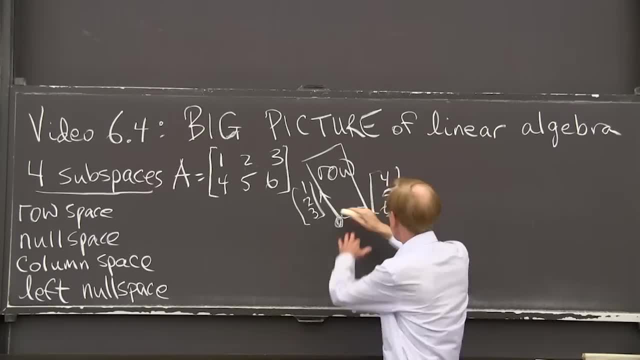 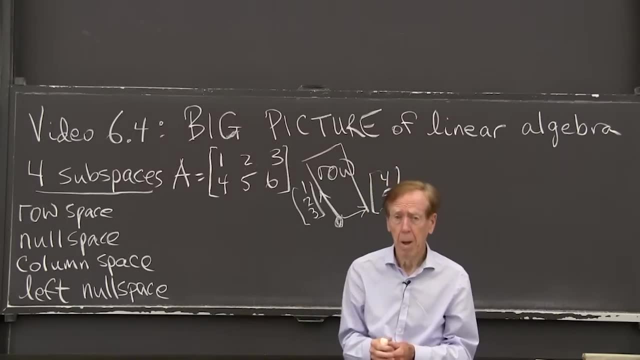 4, 5, 6.. Those two rows And the plane fills our combinations. Well, I can't draw an infinite plane on this MIT blackboard, But you get the idea. It's a plane And we're sitting in three dimensions. 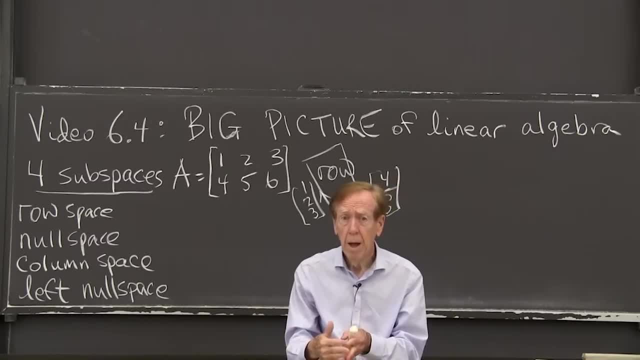 Now the other. so there's more. We've only got a plane here, a flat part like a tabletop extending to infinity, but not filling 3D, because we've got another direction And in that other direction is the null space. 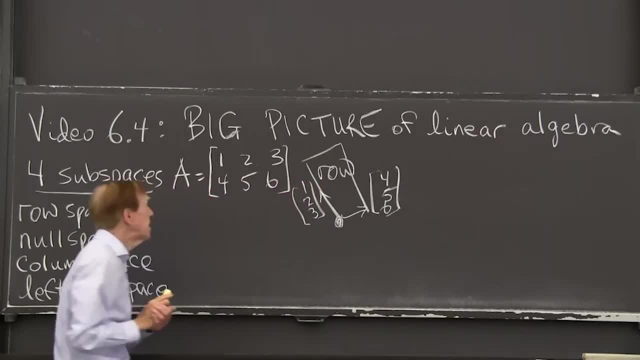 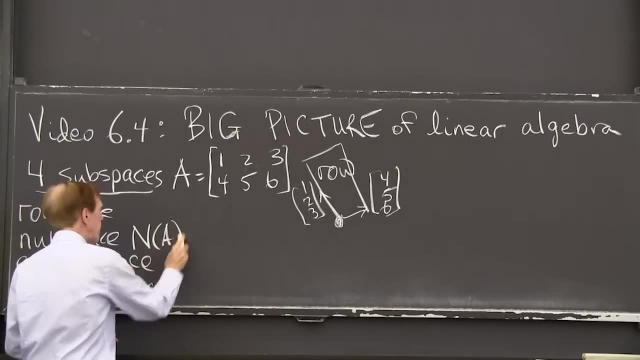 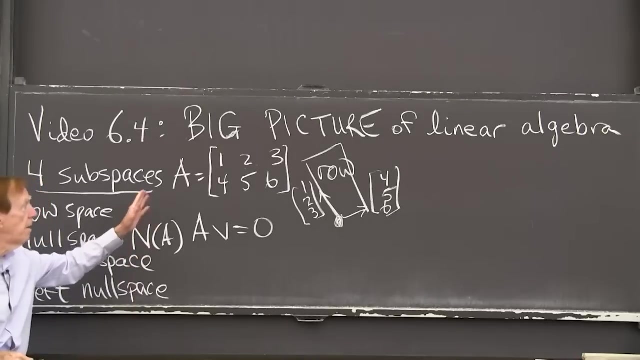 That's the nice thing. So I would like to know the null space of that matrix I'd like to solve. so the null space n of a I'm solving a v equals all 0's, So some combination of those three columns. 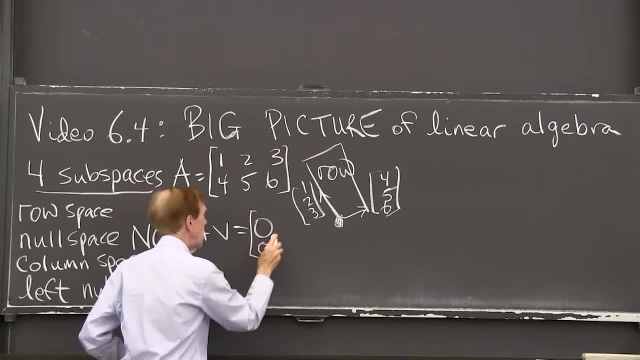 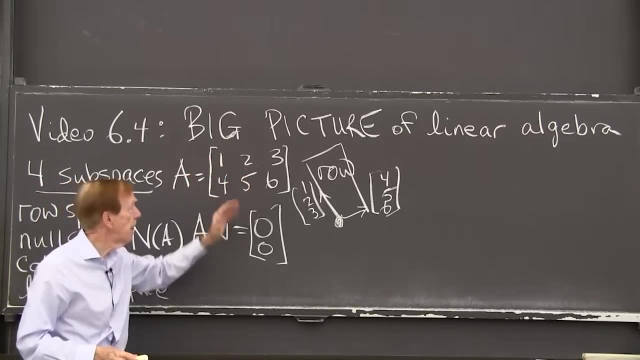 will give me the 0 column. Let me write it in as a 0 column. Let me write it in as a 0 column. What could v be? What combination of that column, that column and that column give 0, 0?. 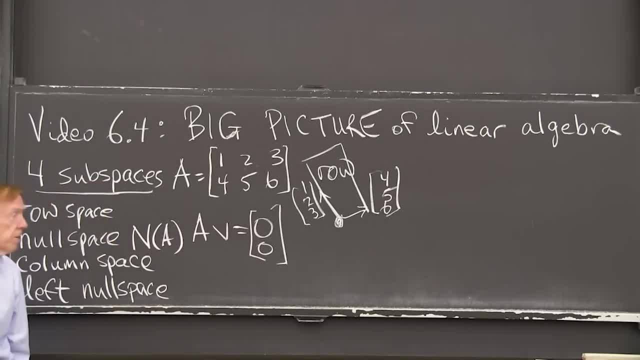 Now I know there are some interesting combinations, Because this only amounts to two equations with three unknowns: v1, v2, v3.. I want to multiply that by v1, that by v2, that by v3. So I have three unknowns. 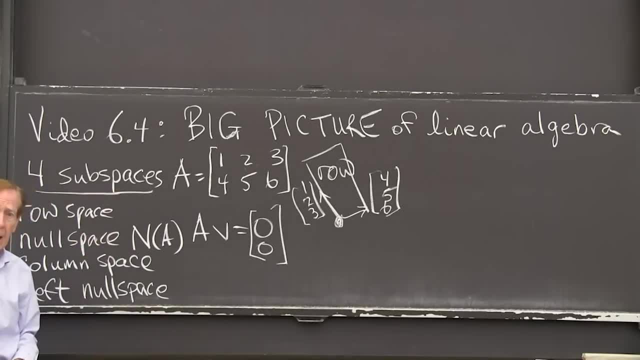 But I have only two 0's to get only two equations. And if I have three unknowns And two equations, There will be lots of solutions And I can see one. Do you see that if I add that and that I get 4, 10.. 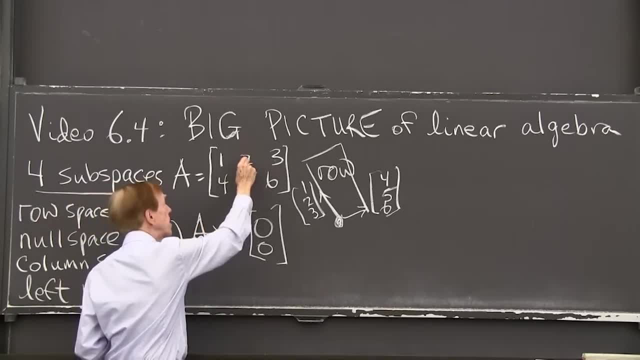 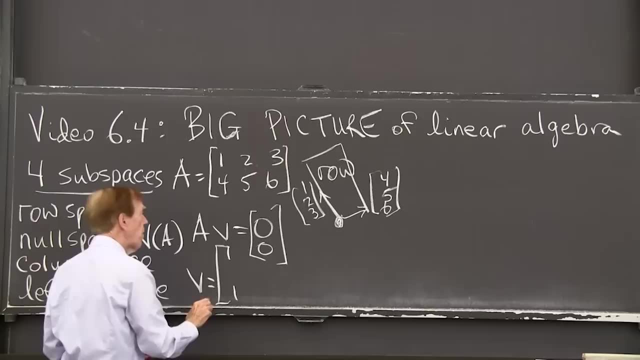 And that's the same. 4, 10 is the same as 2 times 2, 5.. In other words, I believe that v equal if I took one of the first and one of the third and if I subtracted two of the second column. 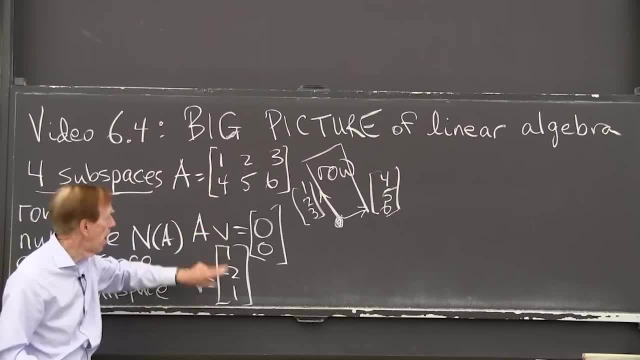 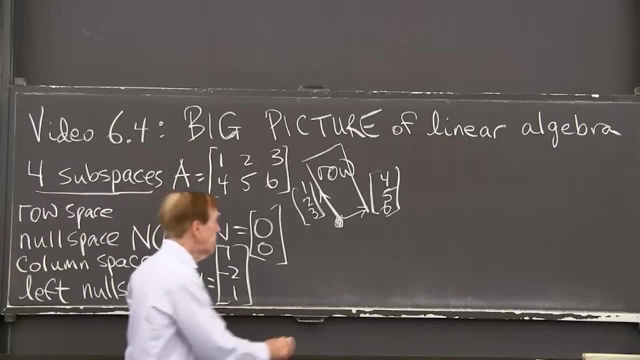 So that Av will give me 1. 1.. 1. 1 of the first column, 1 of the third column And subtracting 2 of the second column will give me 0, 0.. So here's my null space. 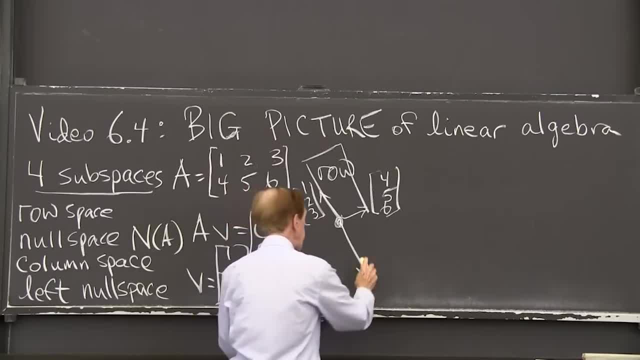 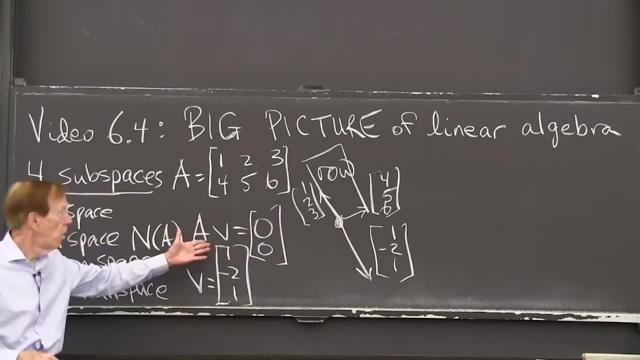 My null space heads off in this direction, in the direction of 1, minus 2, 1.. But of course I get more solutions by multiplying v by any number. 10 times that vector would still give me 0's. 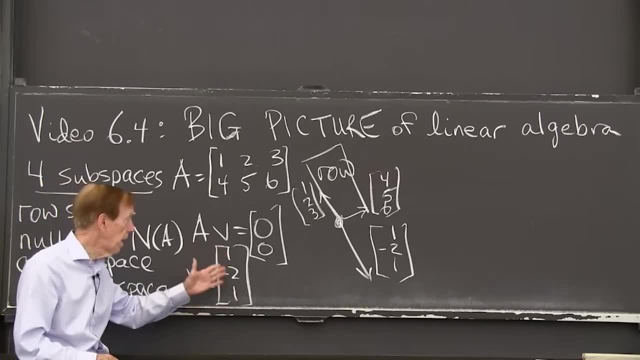 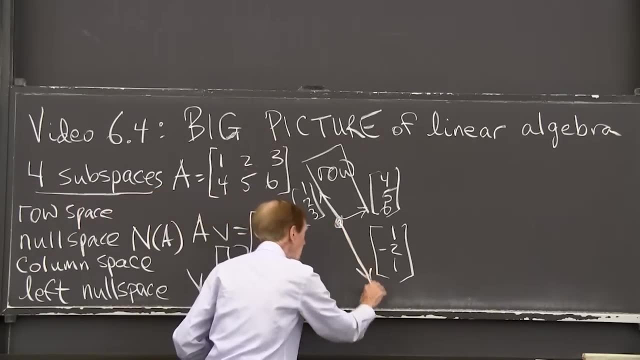 I'll still be in the null space. So I really have the null space as a whole line of vectors. It's that vector and any multiple of that vector. So it's a whole infinite line which is a one-dimensional subspace, The null space. 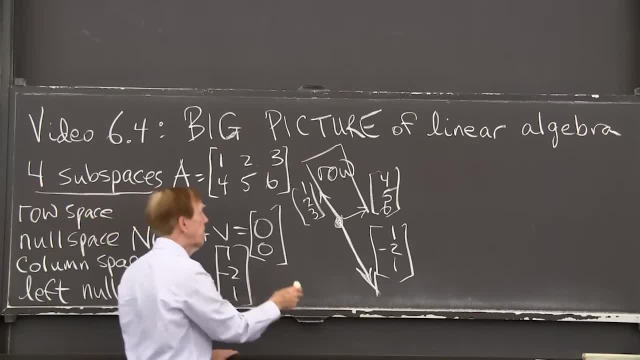 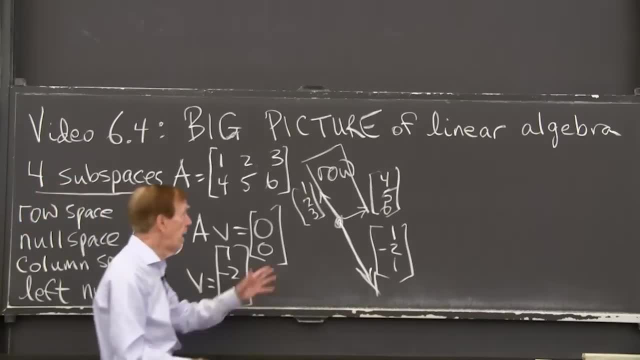 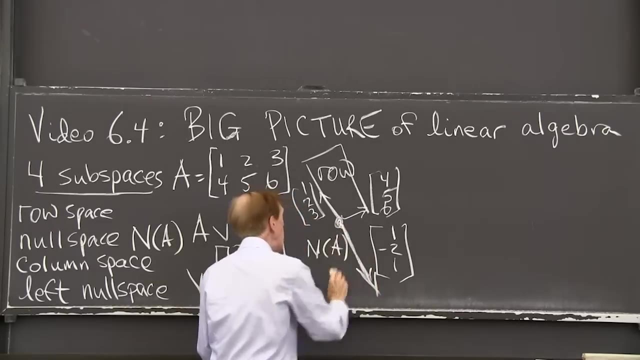 So the null space in my picture. here's the null space. Well, it's not very thick, is it? Because it's just a line. So I'll call this n of a This line. Well, you see, I'm trying to draw a three-dimensional space. 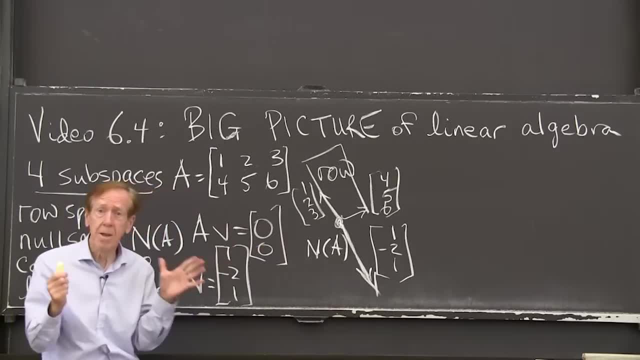 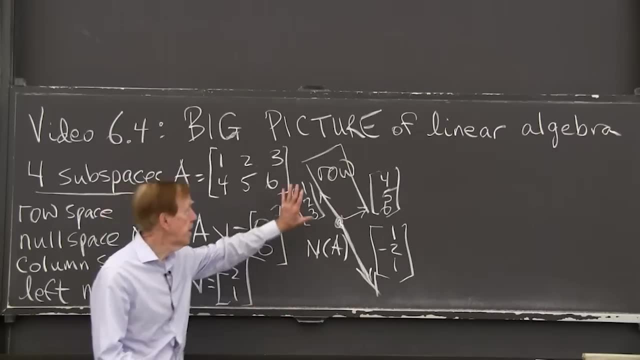 That line goes both ways, But it's perpendicular to the plane. That's the fabulous part. That's wonderful. This line, the null space, is perpendicular to this plane, the row space. You want to know why. You want to just see it. 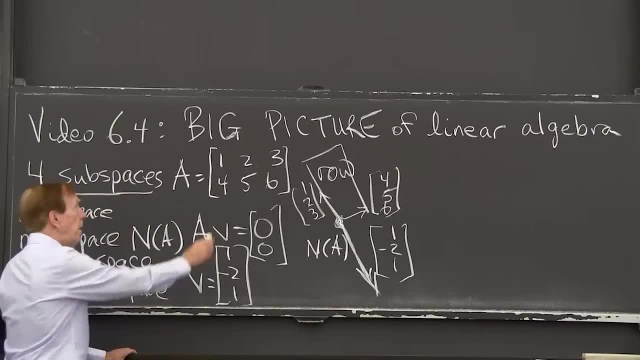 Because if I take a times v, that'll be 1, 2, 3.. Times v 1, 2, 3 is perpendicular to that. How do I check perpendicular for two vectors: 1, 2, 3, dot product 1 minus 2, 1.. 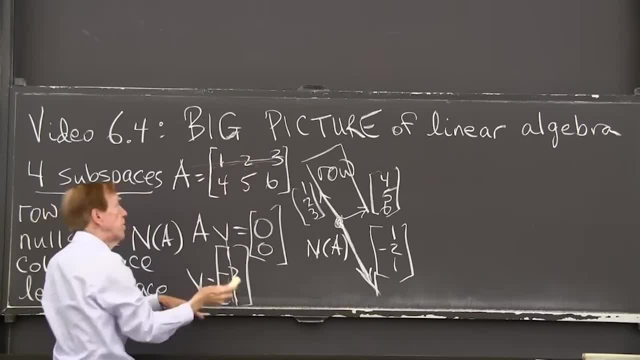 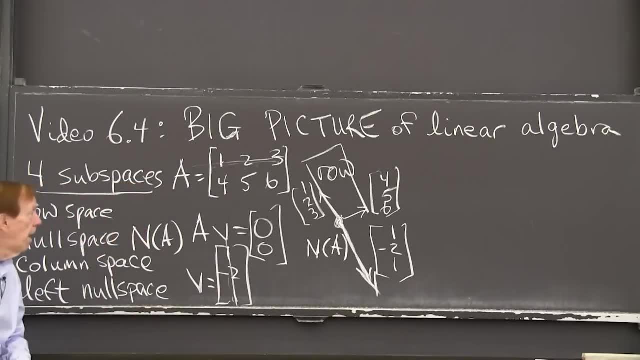 The dot product is 1 times 1, minus 2 times 2, that's 4, plus 3 times 1, that's 3.. 1 minus 4 plus 3 is 0.. And similarly, 4 minus 10 plus 6 is 0.. 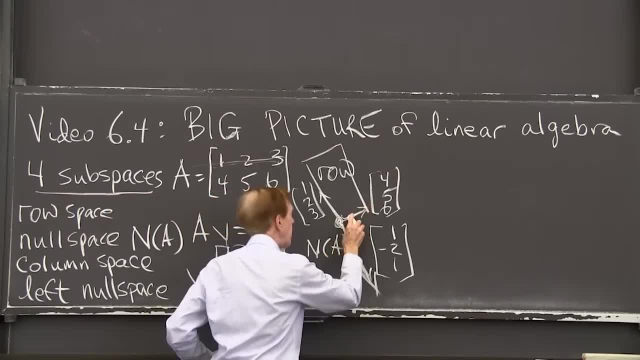 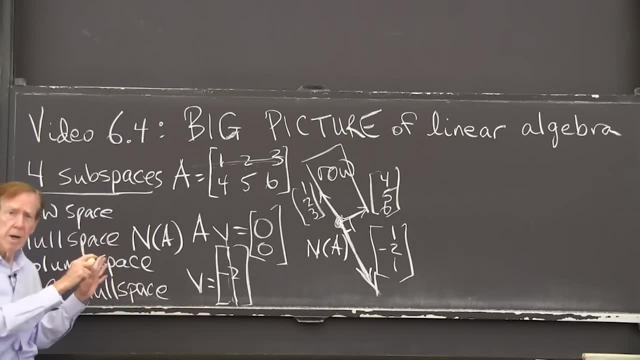 So this is a right angle. here It's a right angle. Right angle: 90 degrees between those two subspaces And again in this example, one space is two-dimensional, a plane, The other space is one-dimensional, a perpendicular line. 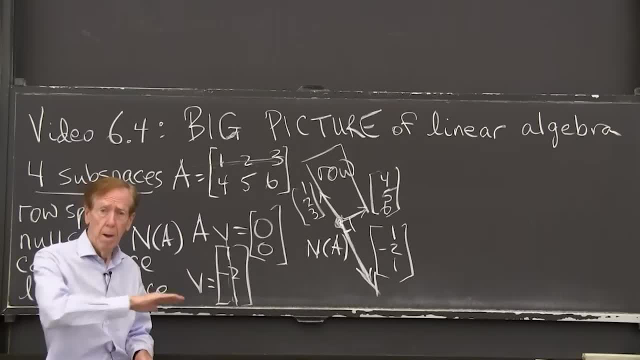 I can show with my hands, but I can't draw on this flat blackboard. I have the plane going infinitely far And I have the line going perpendicular to it And meeting, of course, at 0, at the 0 vector. 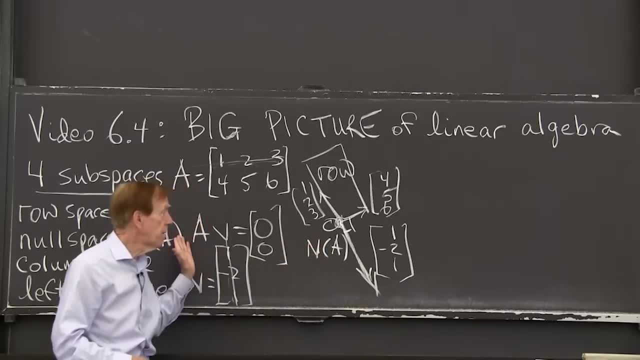 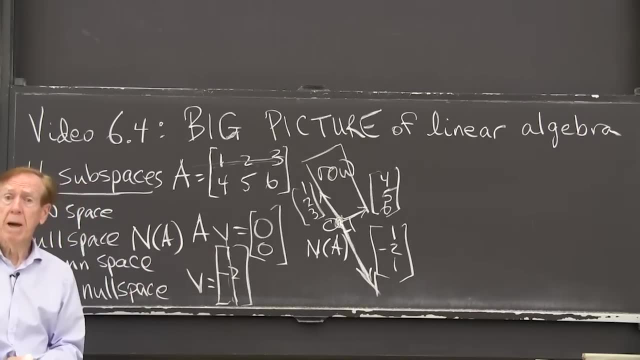 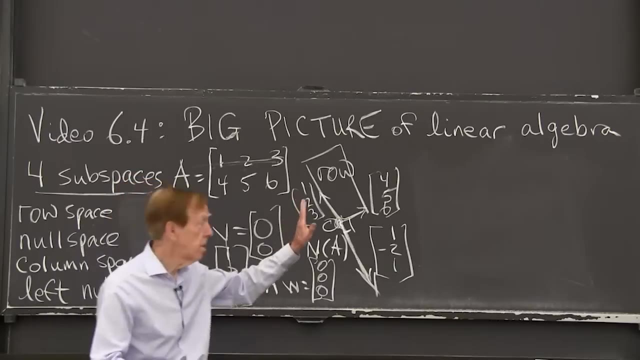 That solves: Av equals 0. And it also it's a combination, a 0 combination of the rows. That's half the big picture: the row space and the null space. Now I'm ready for the other half, which is a second side. 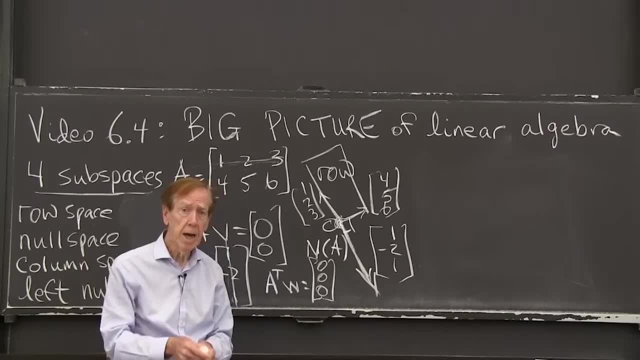 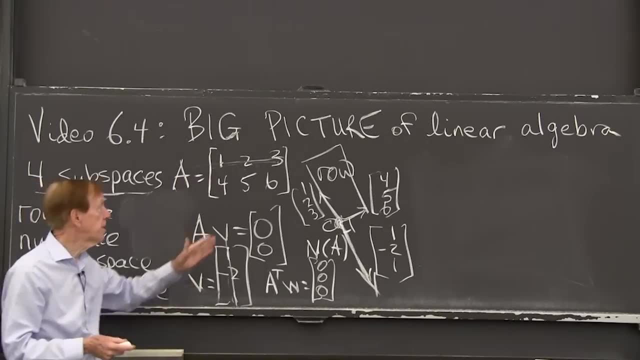 The right-hand side of the big picture contains the column space first of all. So what's the column space of that matrix? So the column space of a matrix. We take all combinations of those three columns, OK So, and that will fill out a space. 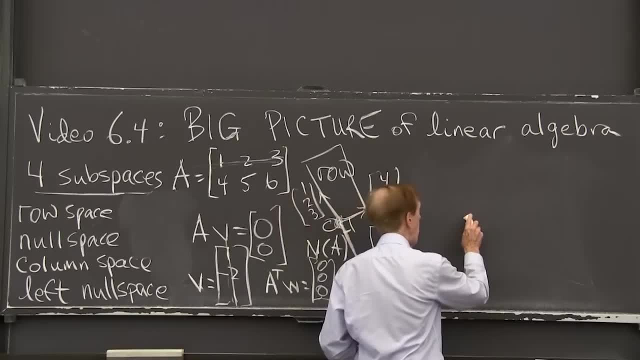 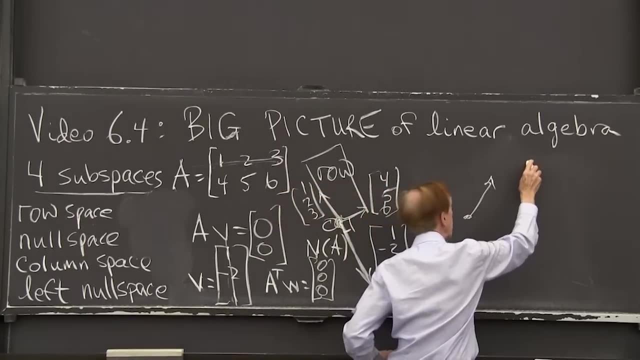 Now I have. so I take the vector 1,, 4,, 1,, 4. And I take the vector 2,, 5, maybe there, And then I'm going to also take the vector 3, 6.. 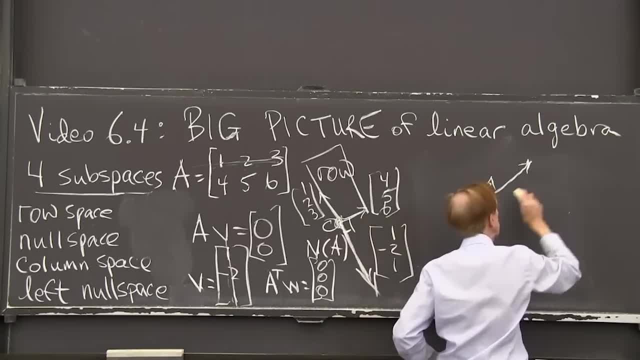 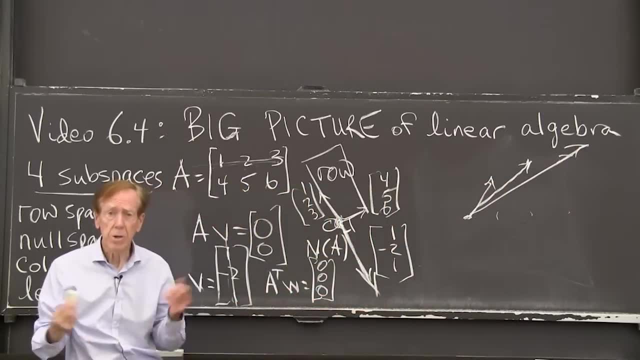 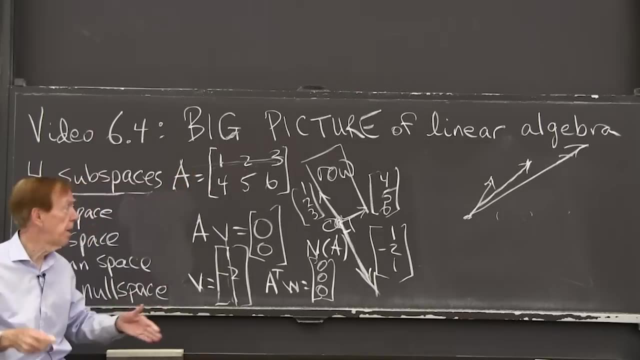 Well, I've got three columns, so I'm counting out 3, up 6.. Good, Take those combinations of those vectors and what do you get? This is a picture in two-dimensional space, because these columns are in two dimensions: 1, 4,, 2, 5,. 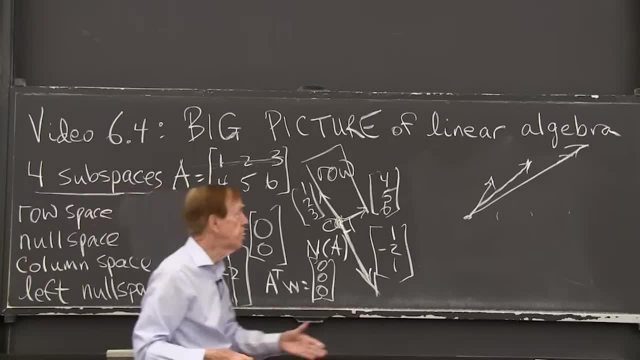 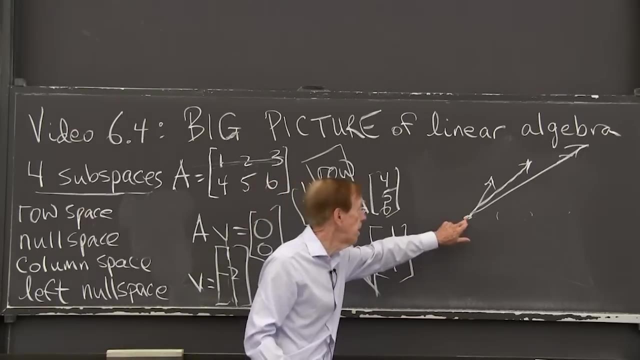 and 3, 6.. OK, When I take the combinations of 1, 4, and 2, 5,, those are in different directions. Their combinations already give me all of two-dimensional space, So the column space is the whole space, including 0, 0,. 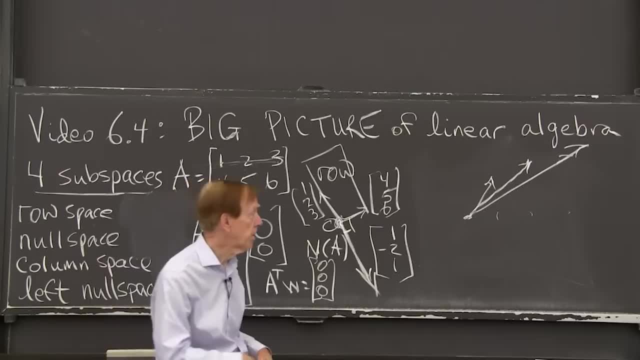 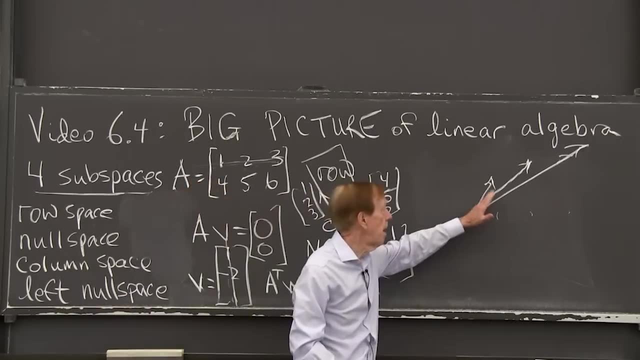 because I could take 0 of 1 plus 0 of the other vector And that third column can't contribute anything new. It's sitting in the column space. It's a combination of those two, But the first two are independent. Their combinations give the whole plane. 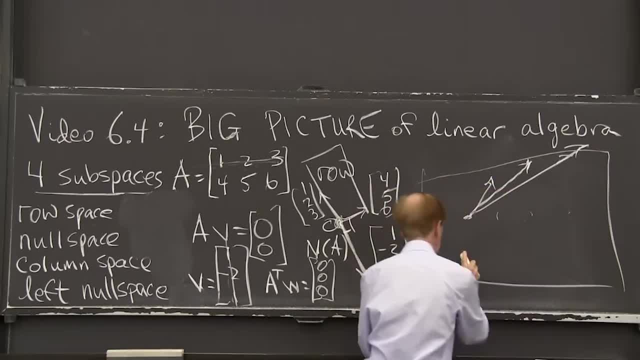 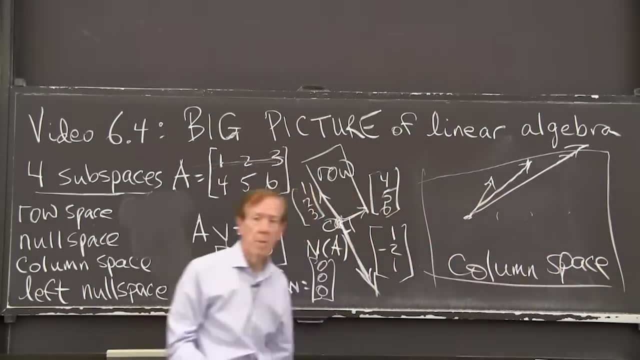 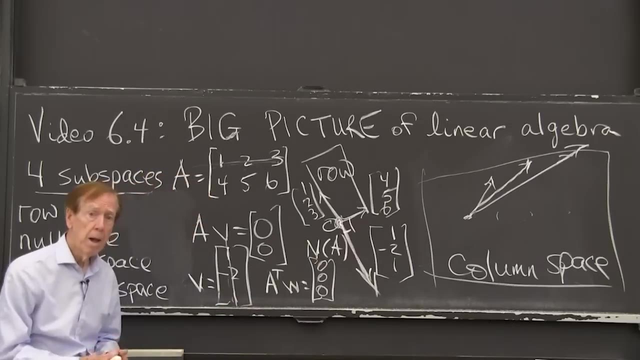 So the column space is the whole plane, Column space. OK, There's not much room for a fourth subspace, But the fourth subspace in this example is quite small. Let me tell you about the four subspaces then. So we know the null space N of A And we know the column. 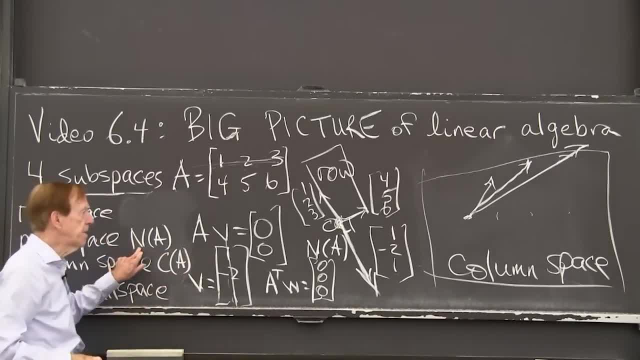 space C of A. The null space was in this picture. The column space was in that picture. OK, Now what's the name for the row space? Well, if I transpose the matrix, the row space turns into the column space, right? 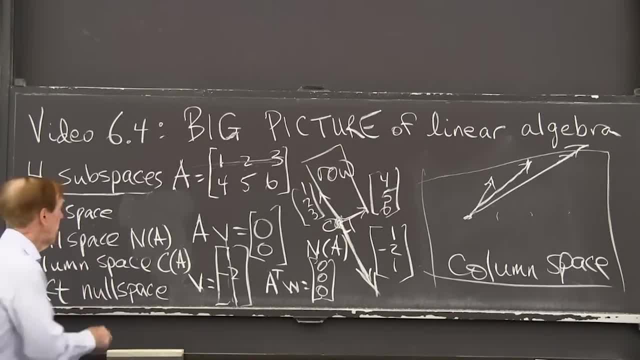 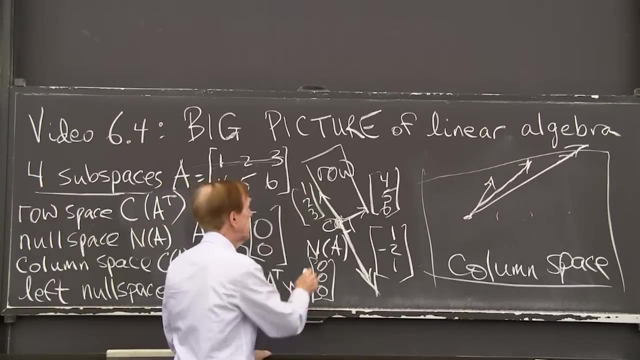 Transpose rows into columns of the matrix A transpose. So by transposing the matrix, it turns these two rows into two columns And that's what I have here. The row space is the column space of the transpose matrix. OK, I like it. 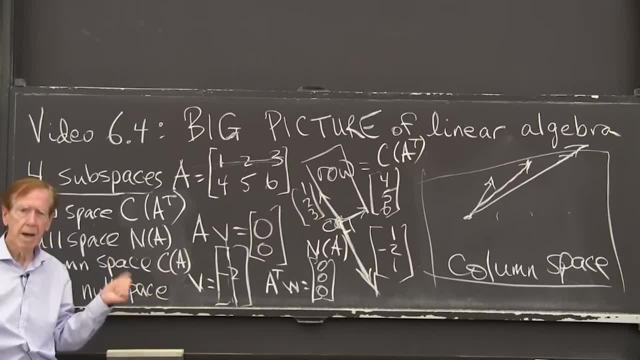 I don't want to introduce a new letter for the row space. I like having just column space and null space And I'm OK to go to A transpose Right Now. what's that fourth guy? Oh, just by beautifulness. General principles of elegance here. 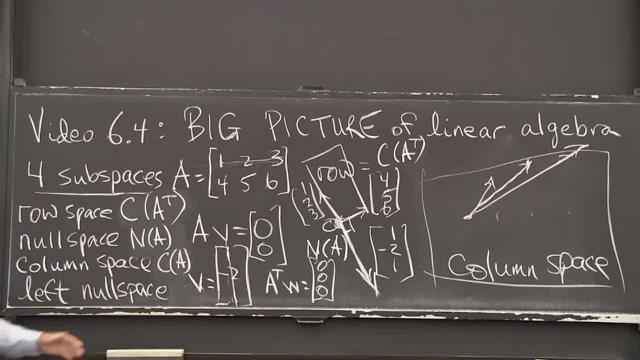 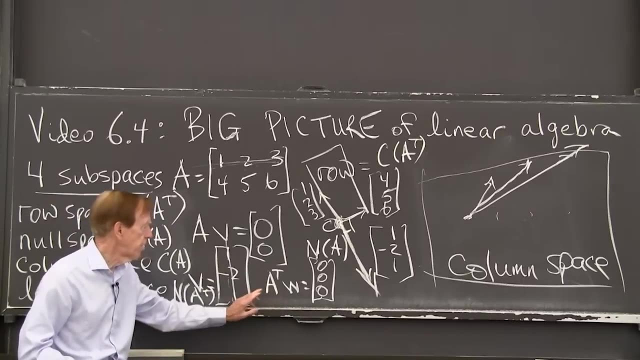 If I have column space and null space of A and if I have column space of A, transpose, the fourth guy has to be: OK, The null space of A- transpose. Sorry, I wrote that so small, So small, But I did write this a little larger. 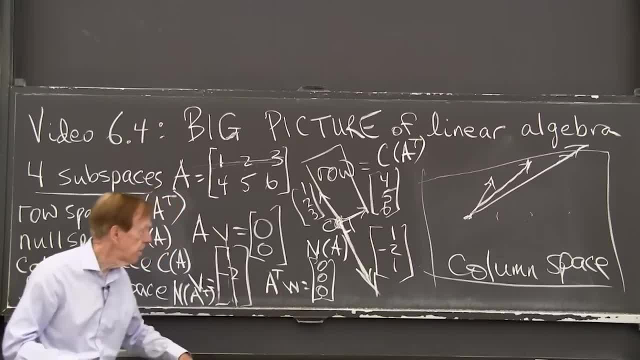 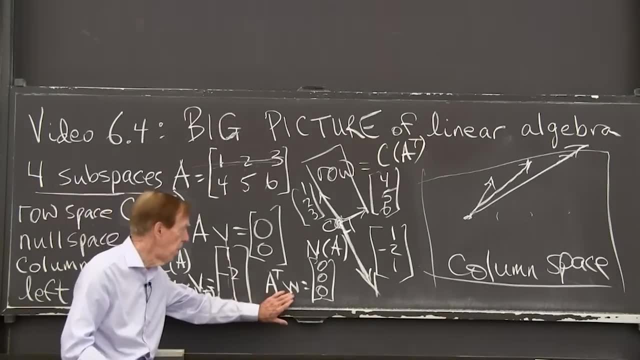 The null space of A transpose all the w's that solve that equation. A transpose w equals 0.. The null space of A transpose is all the w's that solve that equation. OK, What does that equation look like? Ha Well. 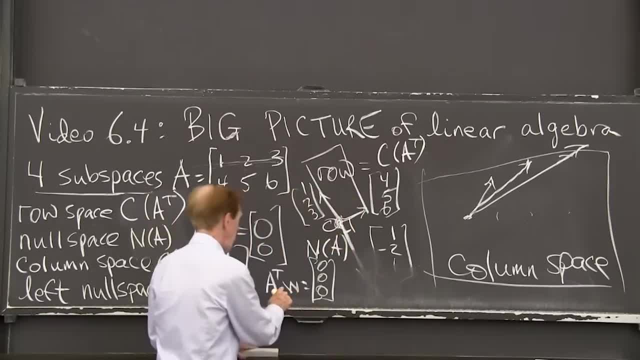 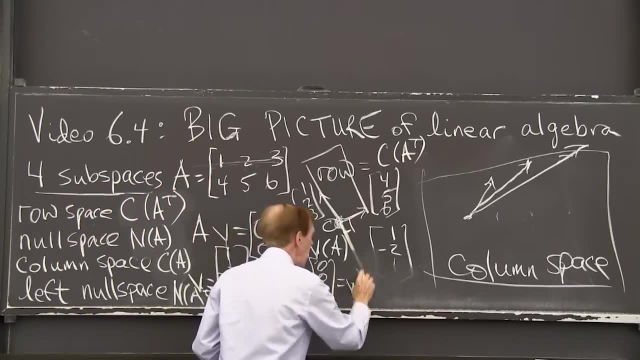 Yeah, Yeah, Yeah, Yeah. So in that equation A transpose will have two columns. So A transpose, this will be w1 of the first, column 1,, 2,, 3, when I transpose, And w2 of the second column 4,, 5,, 6.. 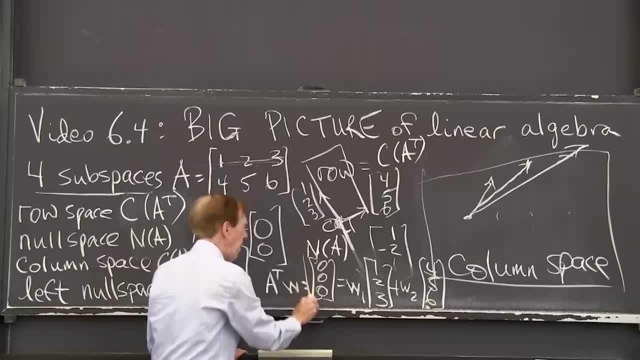 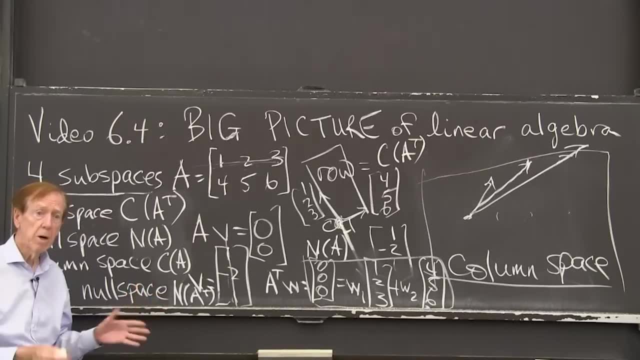 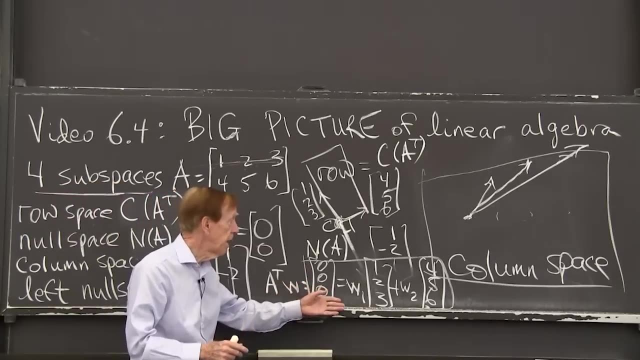 OK, Equaling 0, 0, 0.. Oh Well, Now I've got For this null space, because my matrix here is 2 by 3.. For this fourth subspace I have three equations And only two unknowns: w1 and w2.. 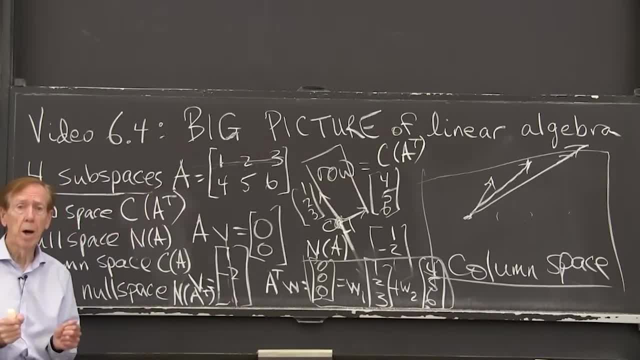 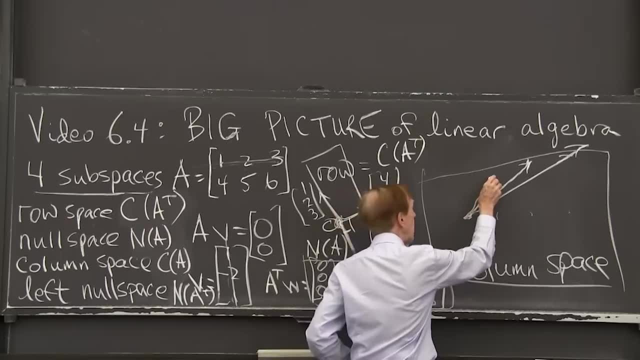 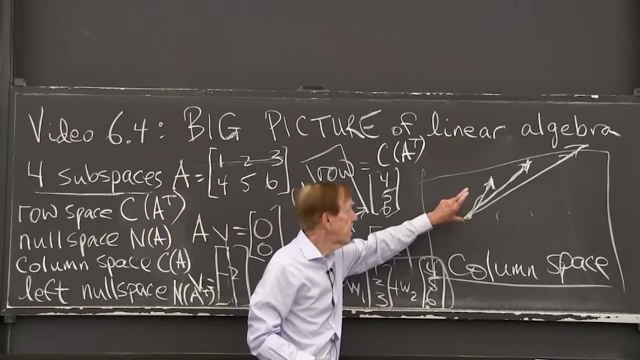 And in fact the only solutions are: w1 equals 0,, w2 equals 0. Because that's the only way I can get, That's the only combination of that vector and that vector that gives me 0, is to take 0 of that and 0 of that. 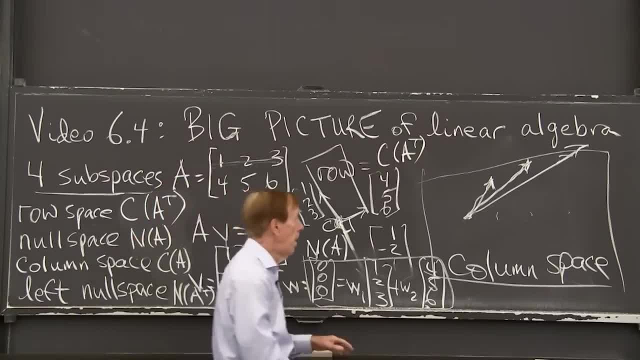 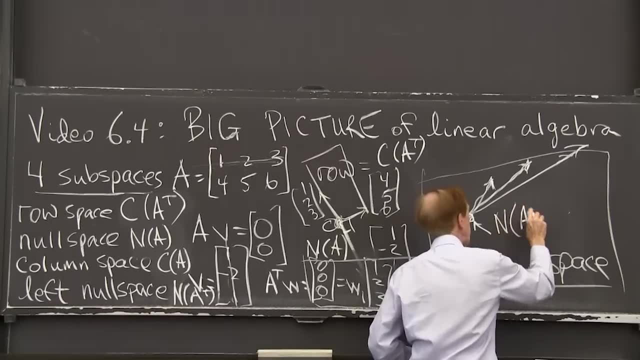 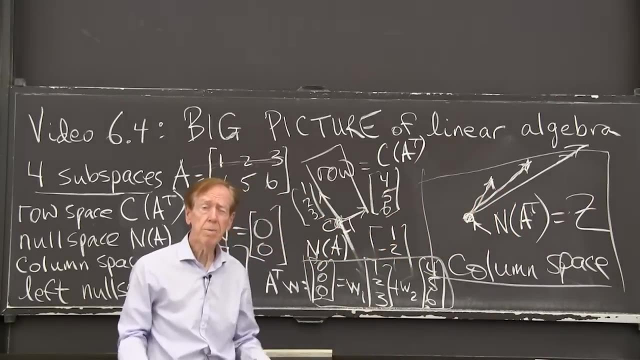 Do you see that in this example, the null space of A transpose is just what I call the 0 subspace, the subspace that has only one puny vector in it, the 0 vector. But that's OK, It follows the rule. 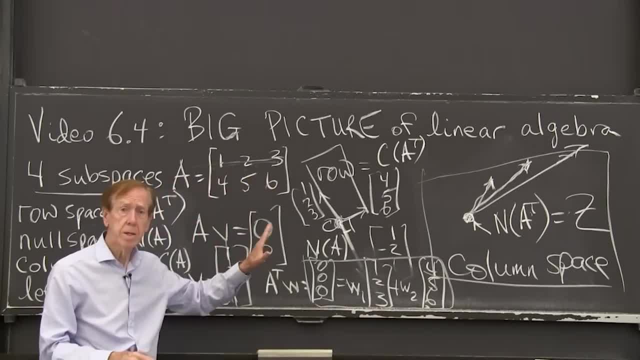 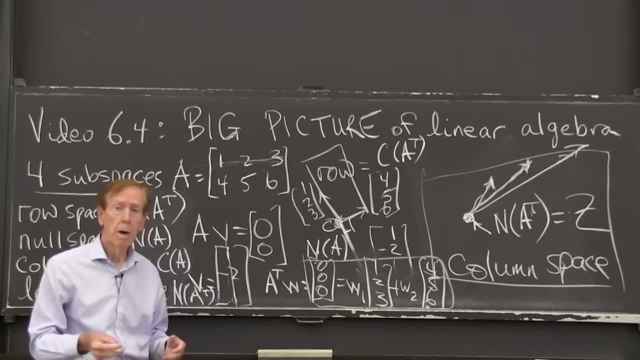 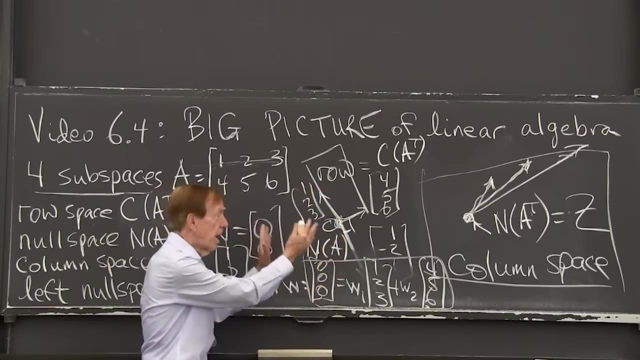 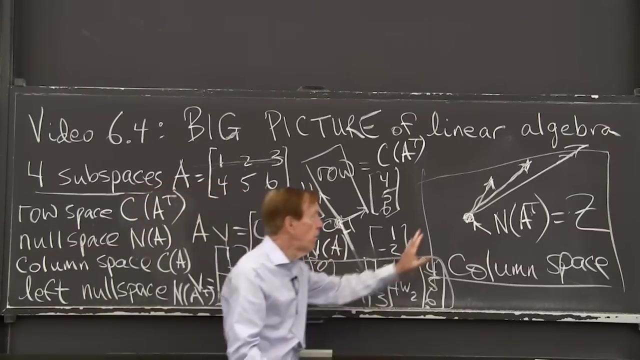 It follows the rule for subspaces And it completes the picture of four subspaces. In other examples we could have all four subspaces, non-zero, But we would have two over here that together kind of complete the full n-dimensional space. And over here we have two that together complete the full m. 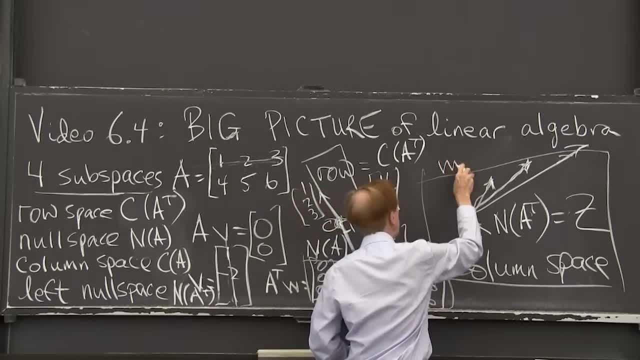 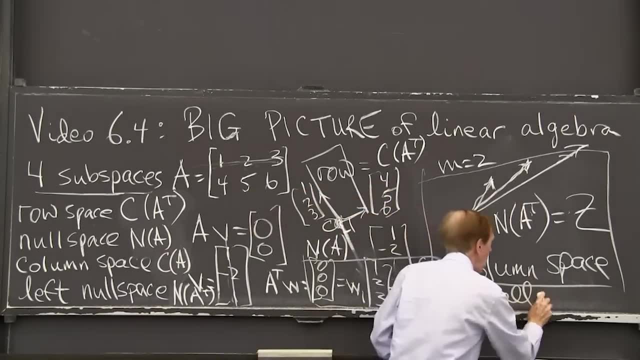 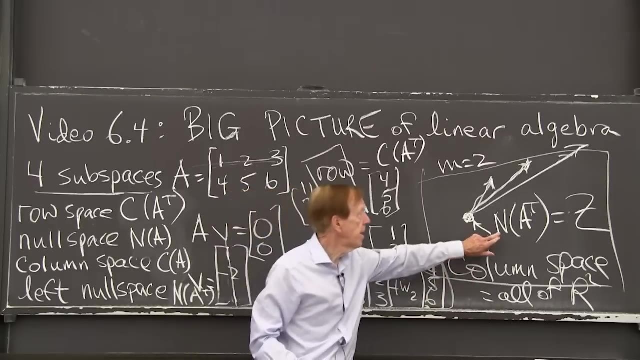 dimensional space, And here for this, matrix m was 2.. So this is completing. The column space was all of R2. in this case, All of two-dimensional space was the column space, And that didn't leave any room for the left null space. 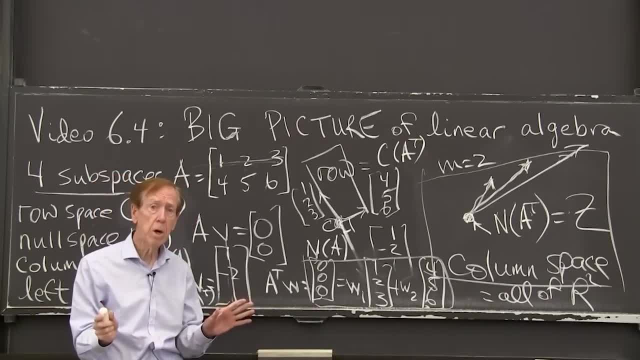 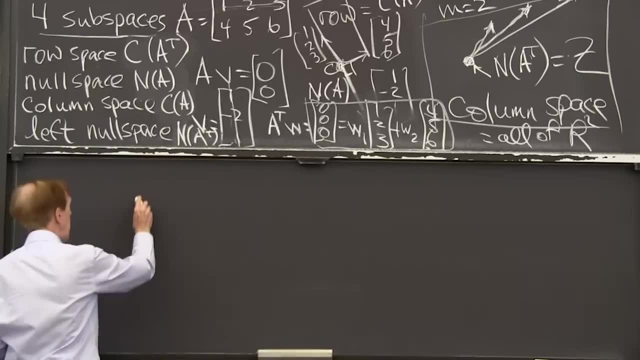 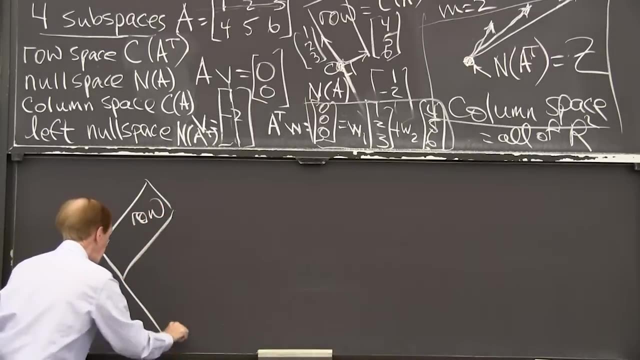 the null space of A transpose. So do you see that picture? Let me maybe just sketch it once more with a clean board. So I have the row space. Let me draw it, maybe going this way: The row space, And perpendicular to that is the null space. 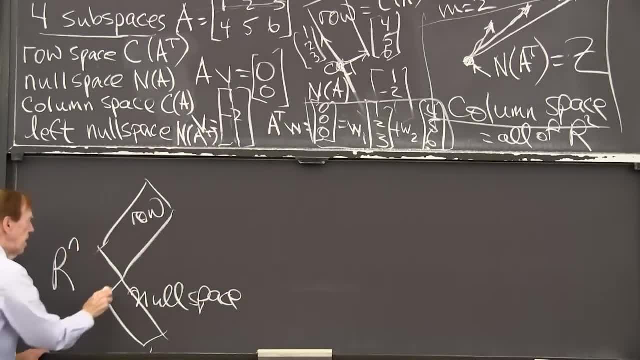 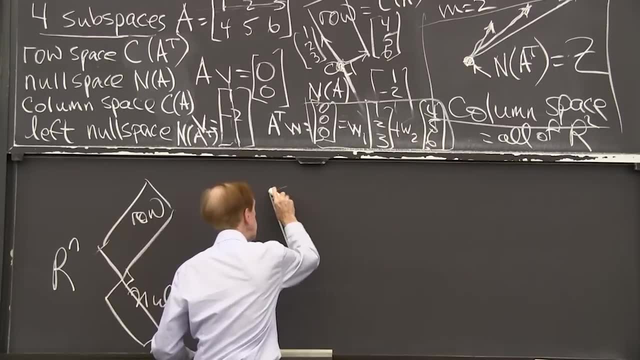 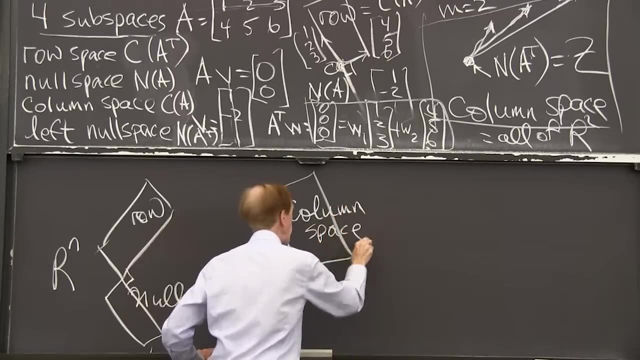 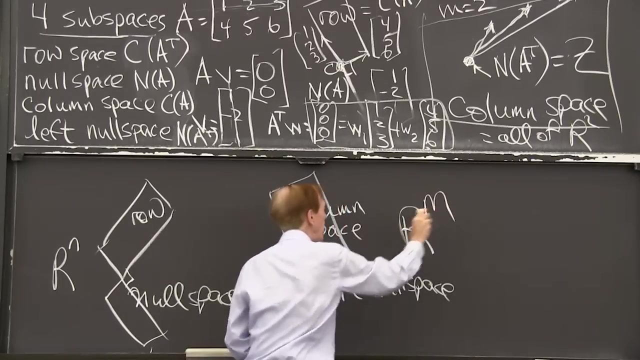 That's in. we're here in n dimensions And they are perpendicular, those spaces. And then over here I have the column space And perpendicular to that is the left null space And we're here in m dimensions. Those are our four subspaces. 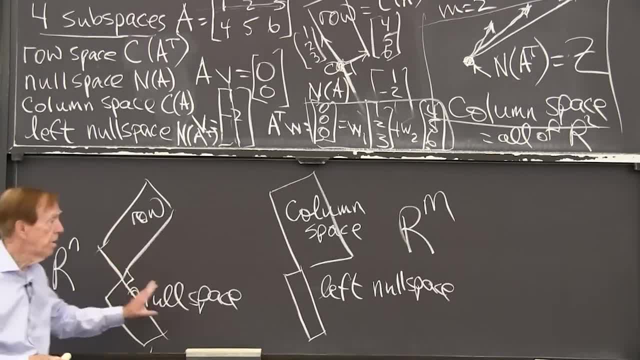 And they sit in n-dimensional space, two of them, Two of them in m-dimensional space, perpendicular, And I could tell you something about their dimensions. So this row space in that example was two-dimensional, It was a plane. In general, the dimension equals, let's say, R, That's. 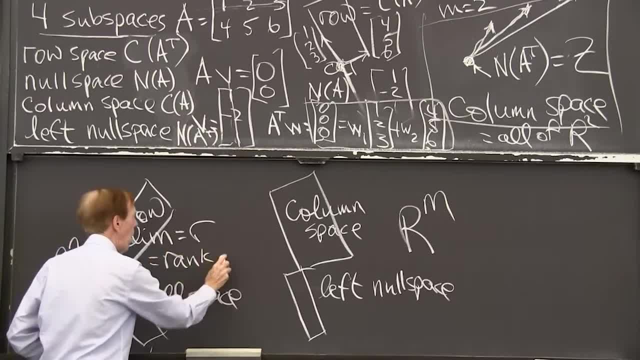 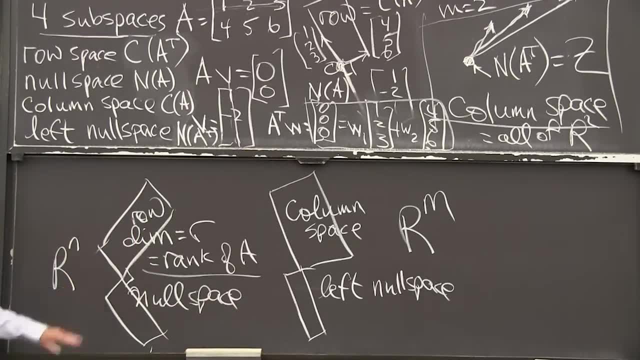 an important number, the rank of A. Oh, that's a key number. Maybe I better speak separately about the rank of a matrix, But I'll complete the idea here. So the dimension of the row space is the number of independent rows. 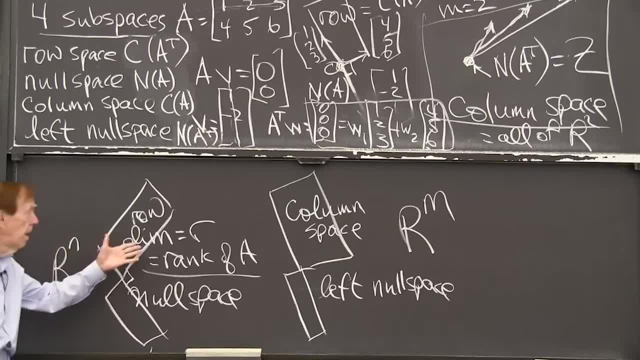 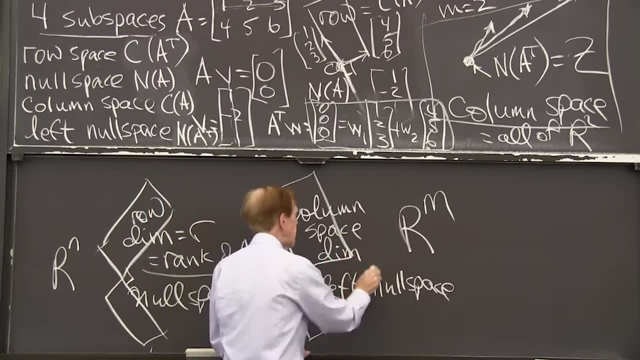 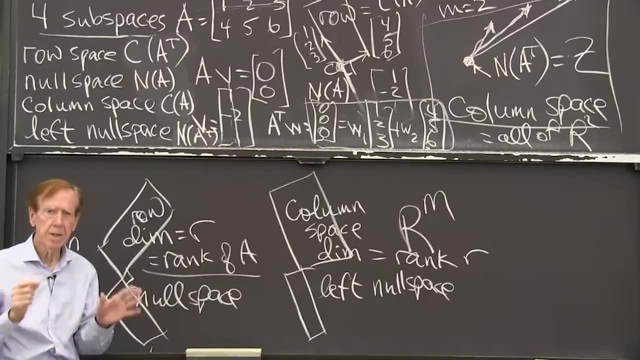 And I call that number R, And the beauty is that this has the same dimension. Dimension is also the rank R. Can I say that Wonderful fact in a sentence? The column space and the row space have the same dimension. The number of independent works on the column space. 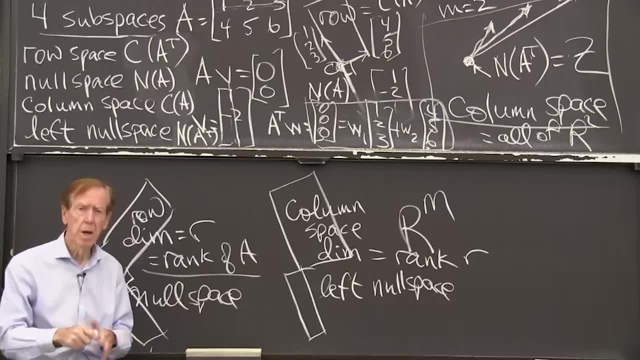 The answer isóc. presenter laughs hours and incidents of ours. The number of independent works on the column space have the same dimension. independent rows equals the number of independent columns. That's like a miracle For a giant matrix. say 57 by 212,. 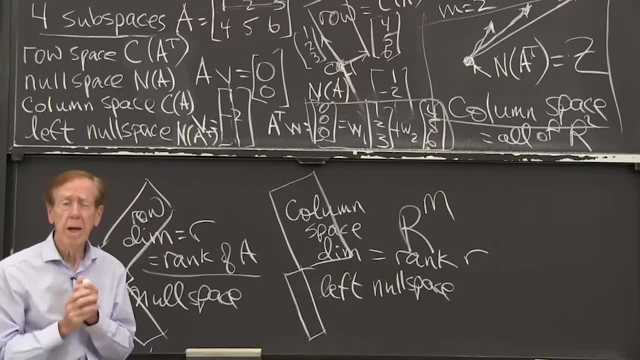 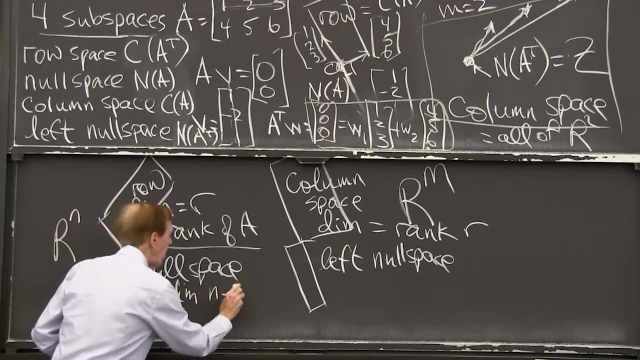 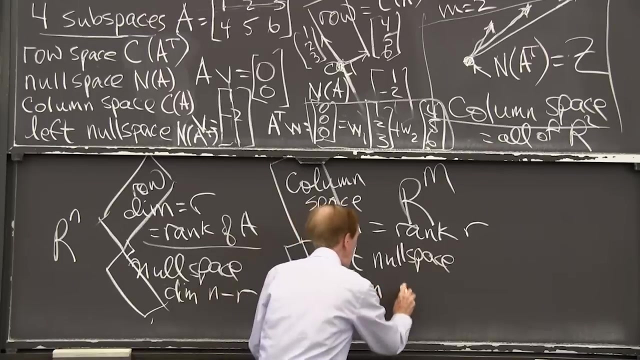 there might be 40 independent rows, Then there would be 40 independent columns, And then the null space and the left null space have the remaining dimension. So the null space has dimension n minus r, because altogether they have dimension m, And this has dimension m minus r. 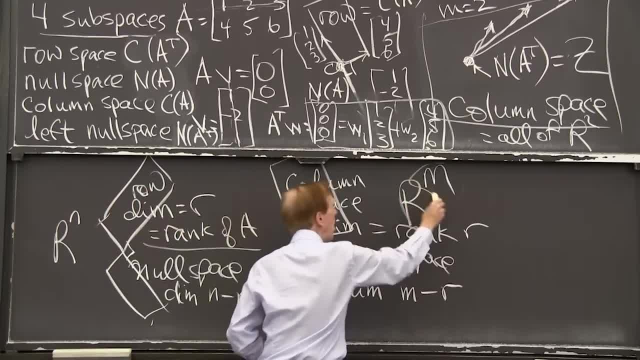 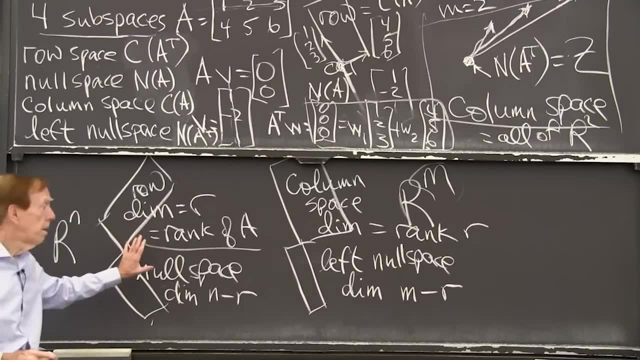 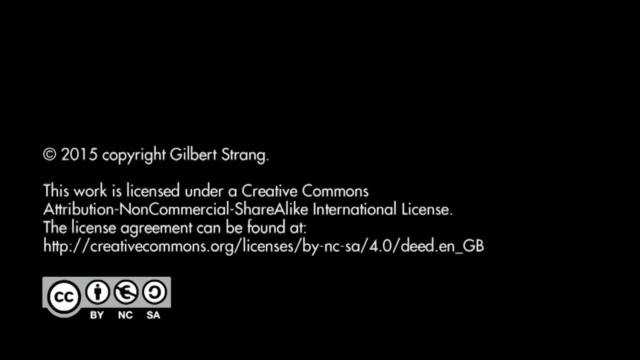 because together they have dimension m. That's the picture with the dimensions put in, And let me say a little more about the idea of dimension in a separate video. Thank you.